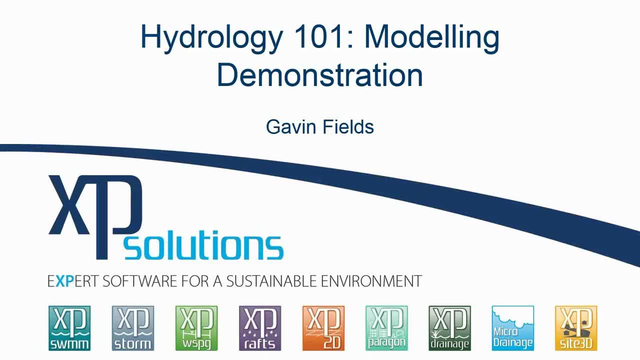 Hello and welcome to today's webinar by XP Solutions, Hydrology 101,- a modelling demonstration. My name is Gavin Fields and I'm a Senior Water Resources Engineer here at XP Solutions. Today's webinar is a follow-on from one of our recent webinars, Hydrology 101, and has been prepared. 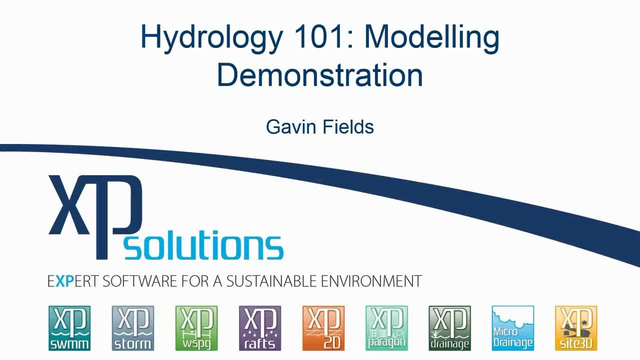 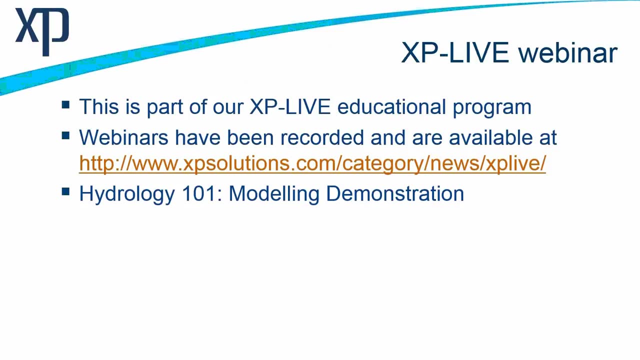 in response to the large number of attendees who are keen to see some practical applications inside the software. pursuant to that previous webinar, Today is part of our XP Live educational program and the webinars are recorded and will be available on our website. Today will be a reasonably short webinar, hopefully. 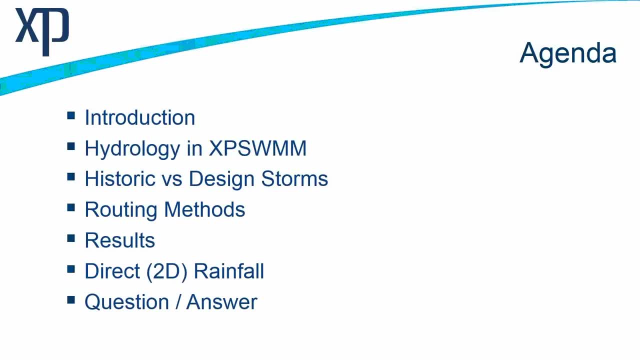 I don't want to take up too much time but as an agenda we'll have a brief introduction, again a follow-on from the previous webinar: discuss the hydrology inside our main tool, XP Swim, and look at the data types between historic and design storms. some routing methods. 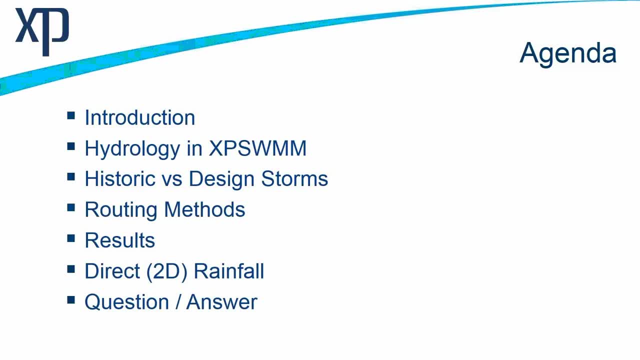 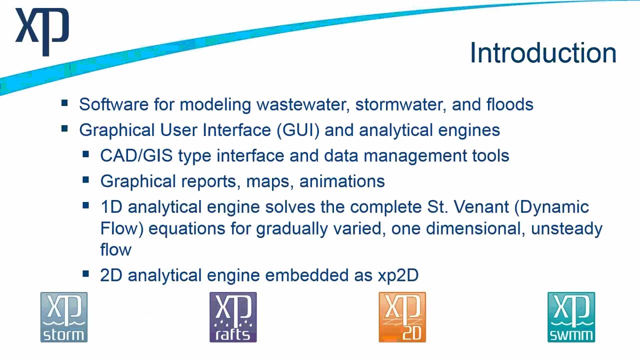 and have a review a lot of the time inside the software for 1D. I'm going to start off with a quick introduction. XP Swim is an engineering tool that models stormwater, wastewater and flooding. It is used across the world and is a graphical user interface with two key analytics: 1. XPSWIM, 2. XPSWIM, 3. XPSWIM, 4. XPSWIM, 5. XPSWIM, 6. XPSWIM, 7. XPSWIM, 8. XPSWIM, 9. XPSWIM, 10. XPSWIM. 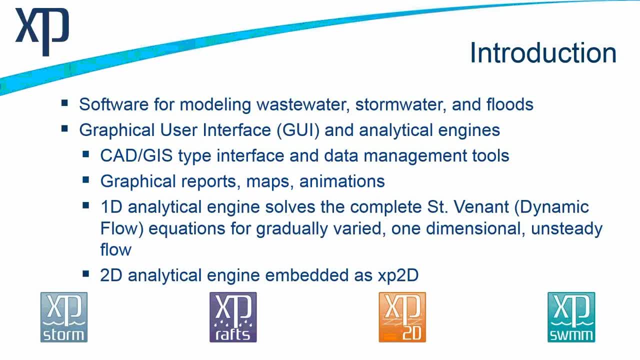 11. XPSWIM, 11. XPSWIM, 10. XPSWIM 11. XPSWIM, 12. XPSWIM 13.. 2. XPSWIM 11. XPSWIM 12. king, 8. XPSWIM, 19. XPSWIM, 18. XPSWIM 13.. 2. XPSWIM 19. xpsw-wim 14. XPSWIM 14. XPSWIM 15. XPSWIM 21. XPSWIM 16. XPSWIM 28. XPSWIM. 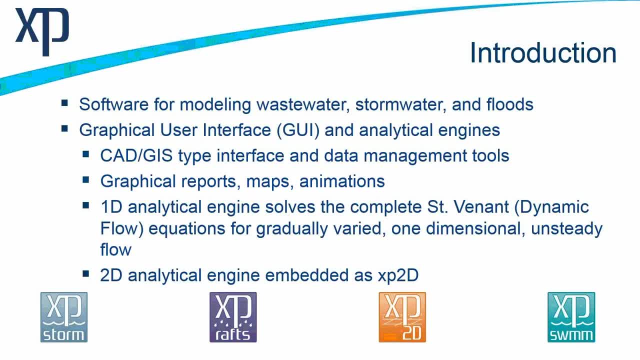 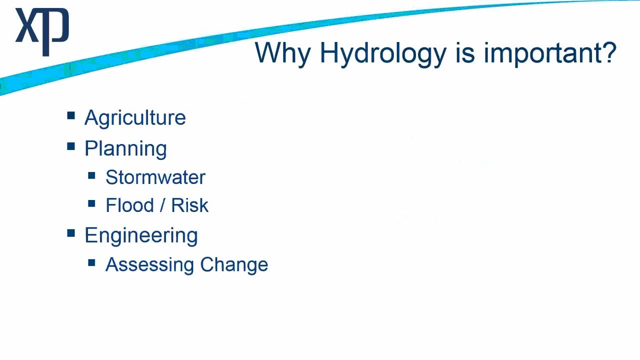 19. XPSWIM 20. XPSWIM, 20. XPSWIM 17.. In actual use, XP Swim will offer missing AD's to� to learn, active, looking, fast seismic data and jellyfish😭. I hope this is helpful to you. 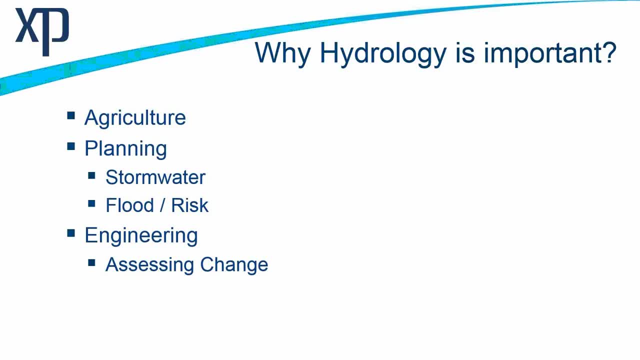 for urban development, residential areas, encroachment points to understand the impacts associated with the land use changes and the subsequent risks associated with flooding. It is also important for agriculture where, in an ever increasing perception of climate change, the demands for our water resources become ever more important. 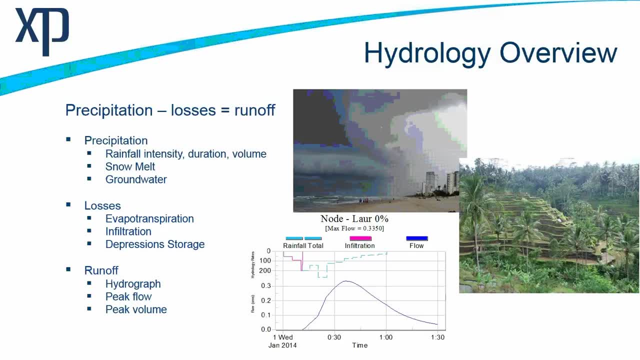 As a very quick overview of hydrology, it is the summation of rainfall minus losses to create runoff. Now, precipitation and the inflows to our hydrology generally come in the form of rainfall, but can also be a result of snow melt and also ground water base flow discharges. 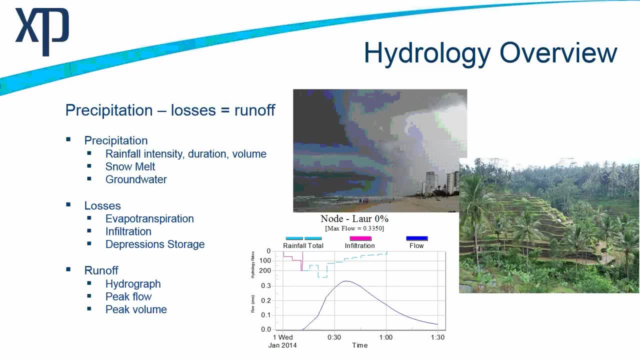 Losses from our models or in the real world In the form of evaporation and transpiration from plants, infiltration into ground water and also surface storage or depression storage. We then try and convert that runoff into hydrographs, as shown in the diagram at the bottom, where 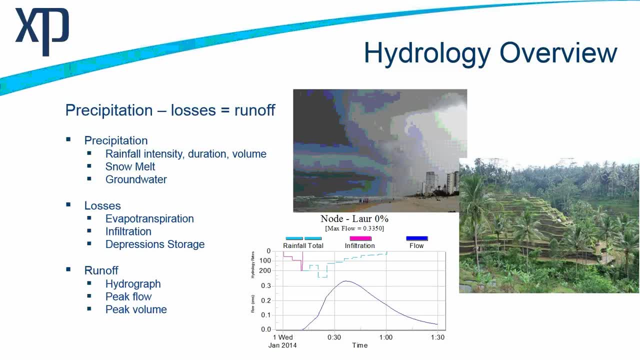 we subtract our infiltration from our inflow rainfall patterns or historical rainfall data to derive a hydrograph and assess peak flows And then at a later stage, which will be part of a future webinar series on hydraulics, convert that to discharge and observe where that flow moves through to. 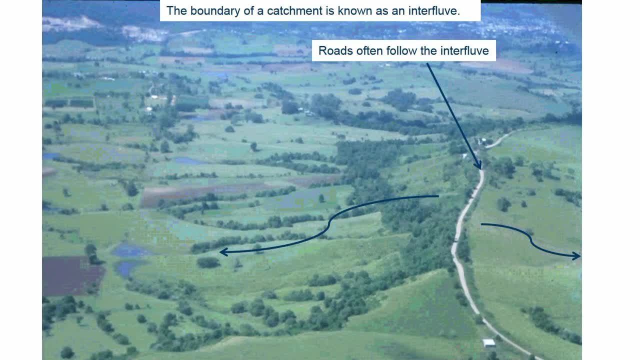 Of course, the first part of hydrology is to understand our catchments. Again, this is taken from our previous slides showing a road along a ridge that is called the interflux, And this is the principal component of hydrology. This is the principal component to start your hydrology assessment: understanding your topography. 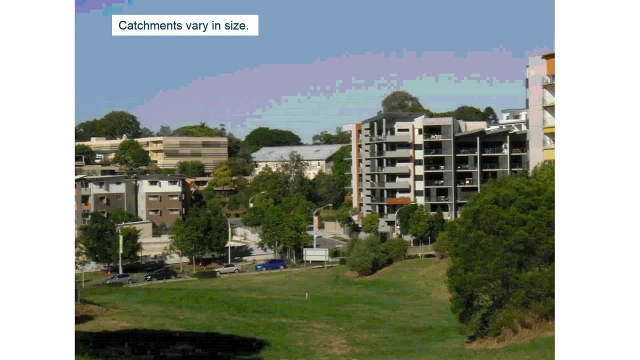 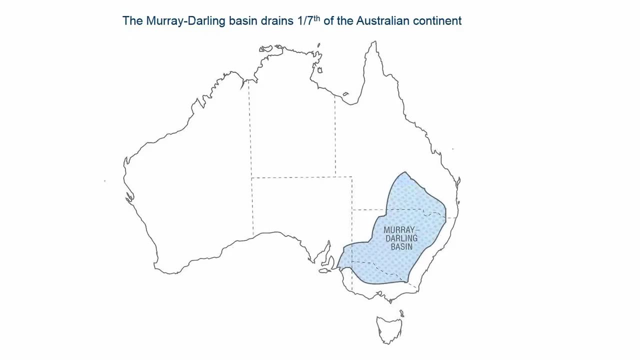 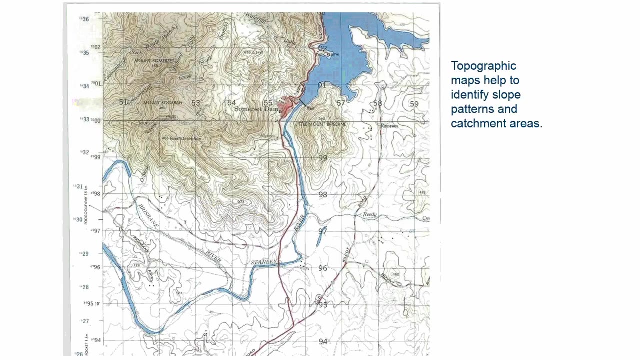 Catchments can vary in size from this small park or to any of the development areas in this particular photo. They can also increase to very large scale basins, such as the Murray-Darling Basin, which covers approximately the seventh of Australia as a singular catchment area. 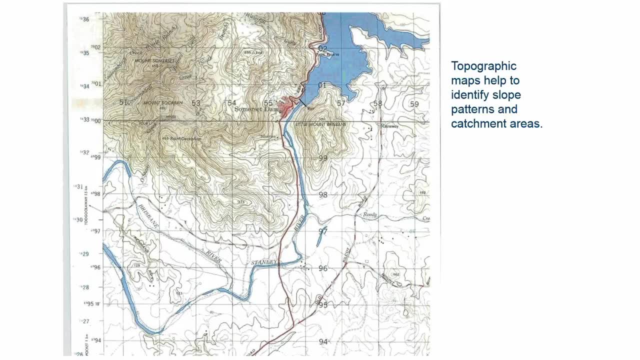 To support us in assessing our catchments, You need to obtain topographic information, whether that be in the form of a detailed survey or historic elevation maps. But that's the first point of contact in preparing your hydrologic model, Moving forward quickly. 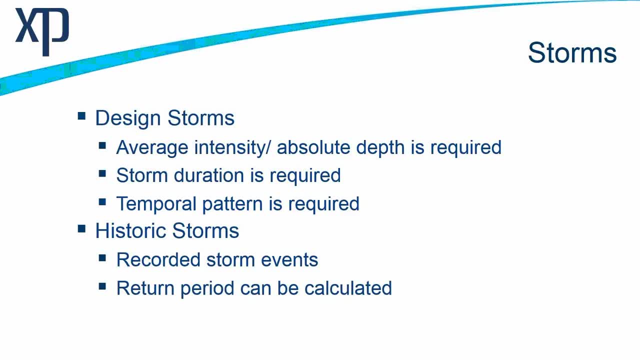 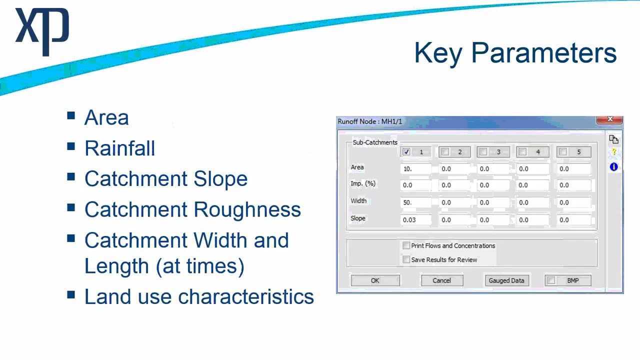 We then have the choice of providing a modelling package, such as XP-SWMM, with design storms or historic rainfall data from your ESP. The key parameters that our software rely upon are quickly summarised here. Obviously, rainfall catchment areas based on those topographic features is number one. 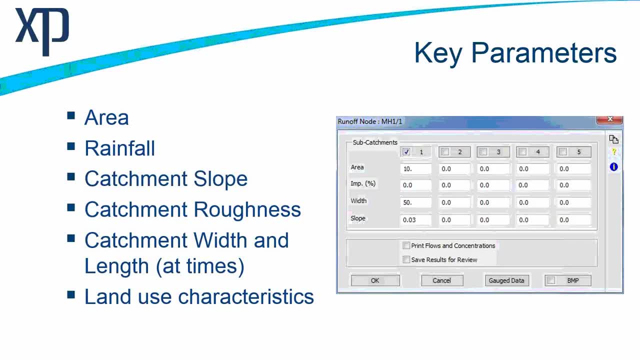 The second point from the data entry perspective in our software is the fraction impervious which is a function of its land use characteristic. Its catchment slope, The roughness of the catchment And, at times, the length or width of the catchment may be important, depending on which method. 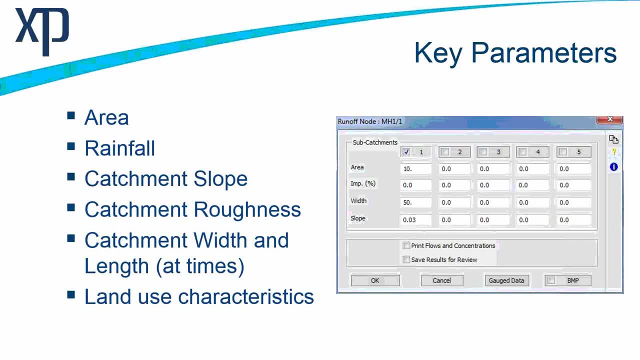 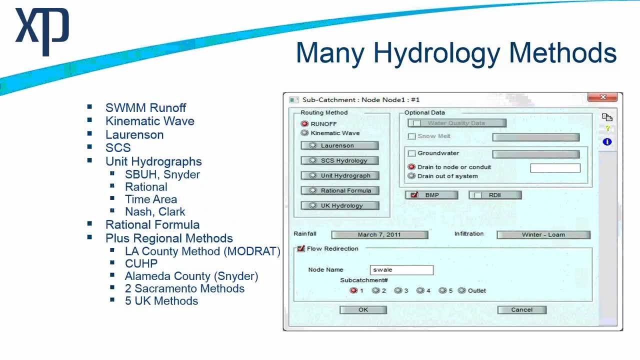 of analysis you are interested in Inside the software. there are many hydrologic methods available to our users. The EPA SWMM runoff method is a dominant method in America. Here in Australia the Lawrencense method is very favoured And across the American and Asian regions the Soil Conservation Service methods would. 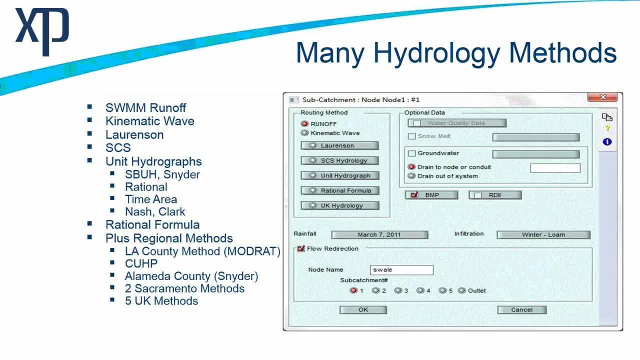 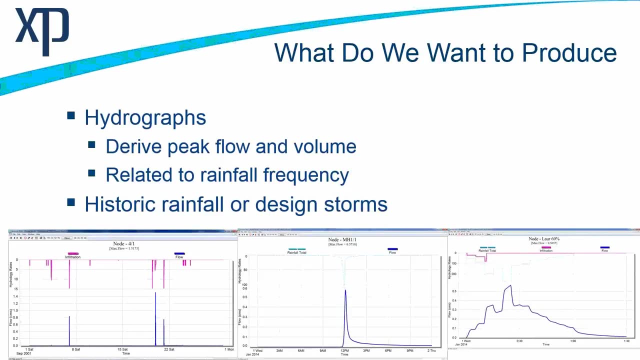 probably be the number two or three method out of most of our user base, And, of course, there are other regional methods that have been prepared for specific areas. And so what do we want to produce? Obviously, we want to understand our peak flows, prepare graphs, some of these at the bottom. 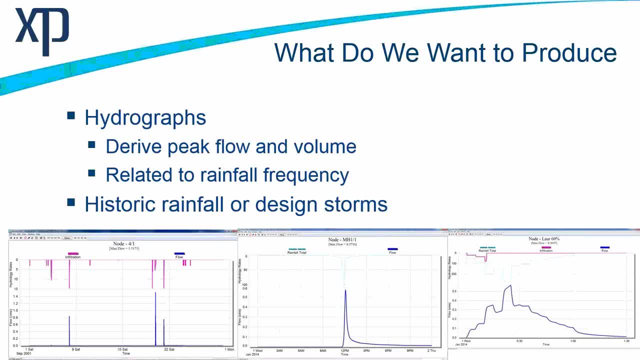 of the screen, To understand the flow, To understand how this data is going to manifest in our list of rainfall or design storms. At this point I'll jump over into the software and we can have a look at the practical applications inside SWEAT. 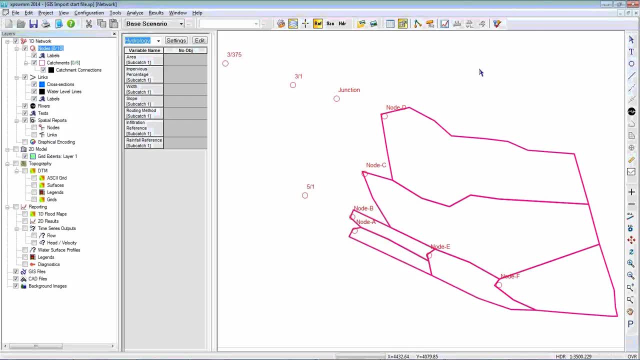 So this is a simple model that is available to all of our potential users. If you are willing to contact us here at XP Solutions, we can provide evaluation versions or trial versions of the software, And these datasets are included for your use. following this session. 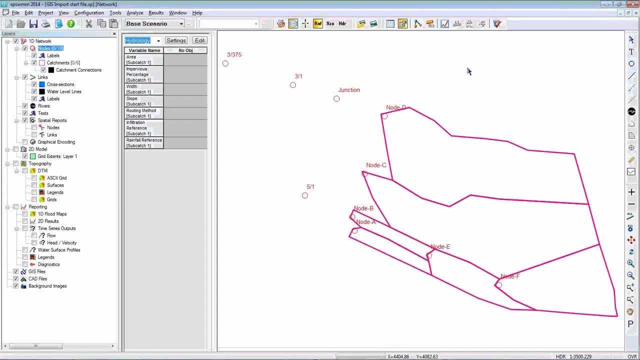 But in this example, I just have a number of nodes and some catchment areas that have been already drawn into the software, And we can link catchment areas that have been drawn manually, which I could do like so to continue to manipulate this, And I can quickly add an additional catchment as required. 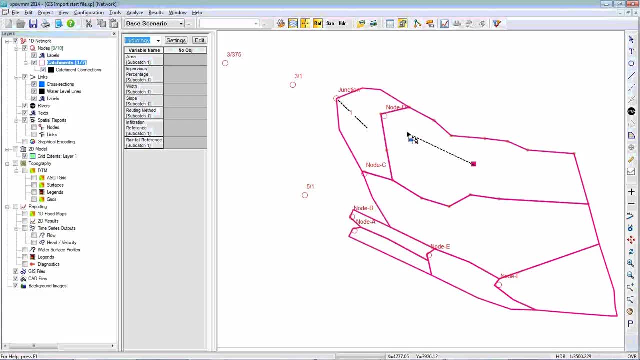 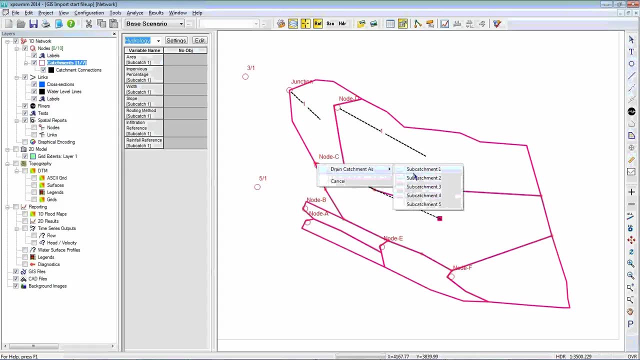 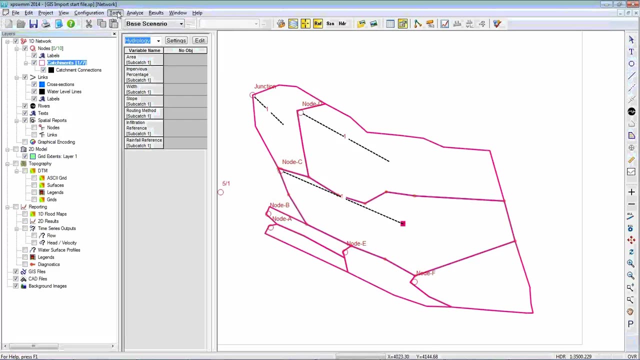 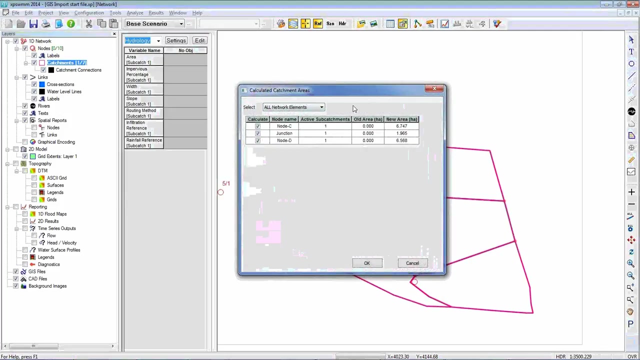 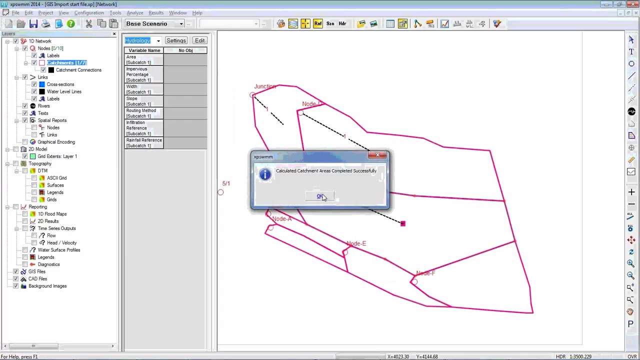 We can link these catchments to our nodes inside our software And we can derive additional information from these polygons very rapidly. Once you've done this for the entire catchment, we can use tools within the software to calculate catchment areas And it will give us a quick report on the elements that I've changed to show that up. 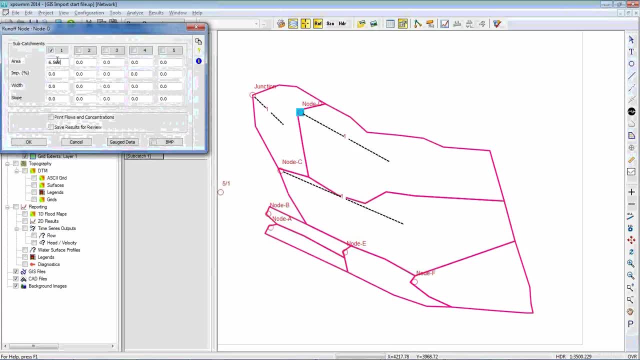 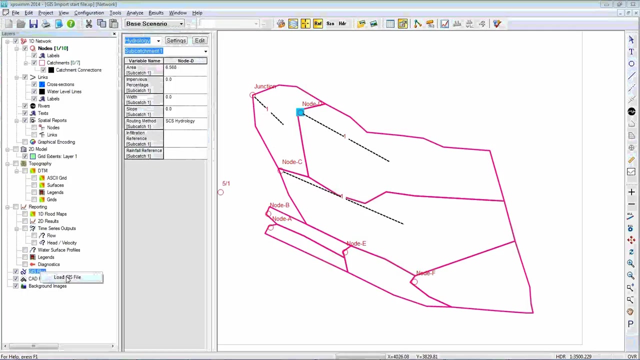 And now, when I click into these elements, I can see that I have the catchment areas that have been applied to the nodes. We can see here that we still need to obtain additional information beyond these elements. If we have a GIS database in the background, I can load catchment information and I have. 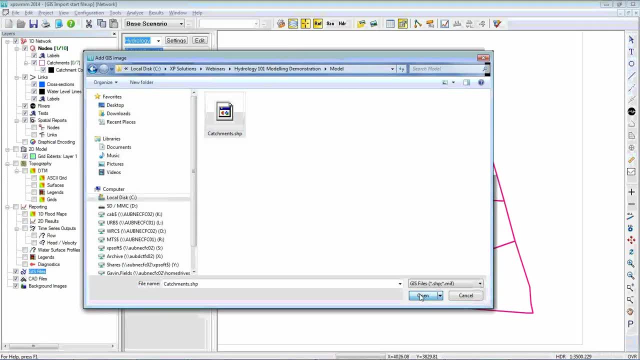 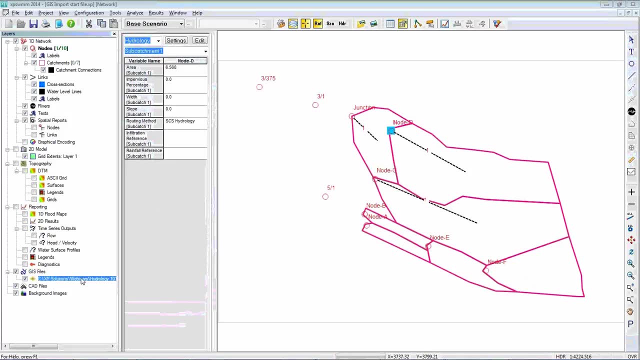 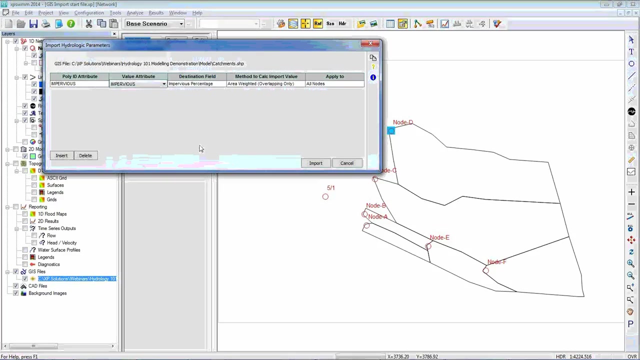 a GIS shape file. Now that I've linked this shape file into the software, I can now actually, if I hide these catchments, I can see that the catchments are available on this GIS file as well. these black polygons: I've right clicked on this layer and then this has brought up this dialog box where 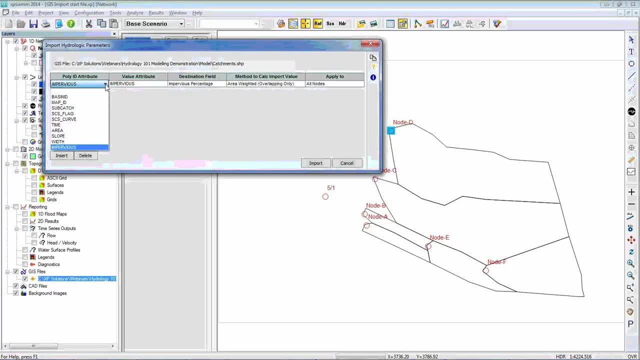 I can select Attributes from the shape file and then apply them to core components of the software. Part of the cookie cutting feature of this element is that if you have multiple polygons with land use information that may include fraction impervious components, then we can. 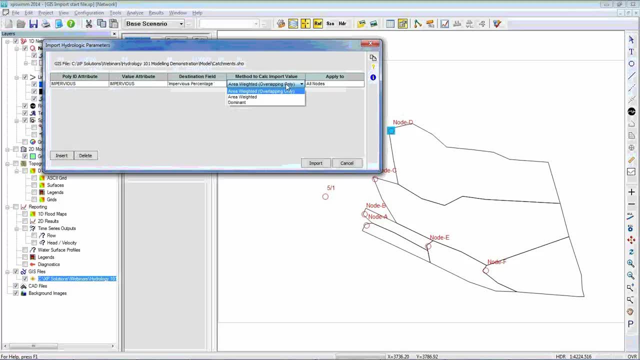 do an area weighted method to derive a final fraction impervious, for example? So if a component of the catchment was used for open space and then residential adjacent, you may wish to get a cumulative fraction impervious that may be as low as 20 or 30%. 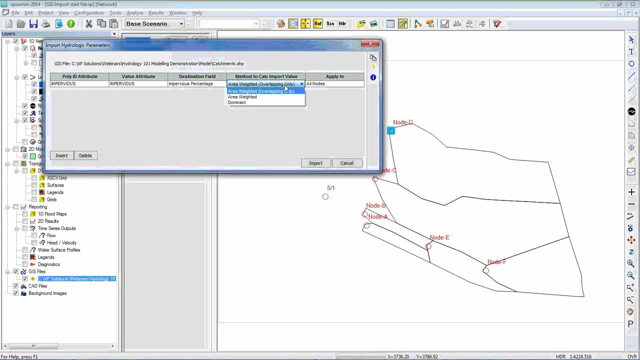 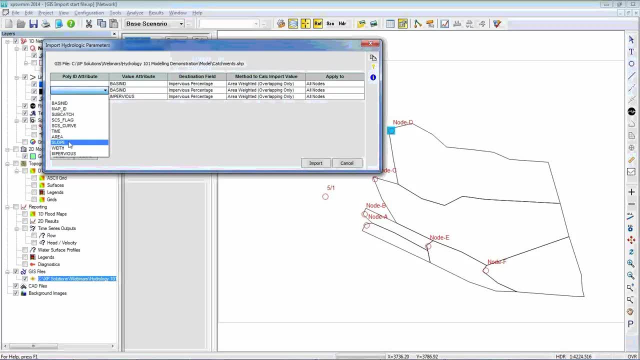 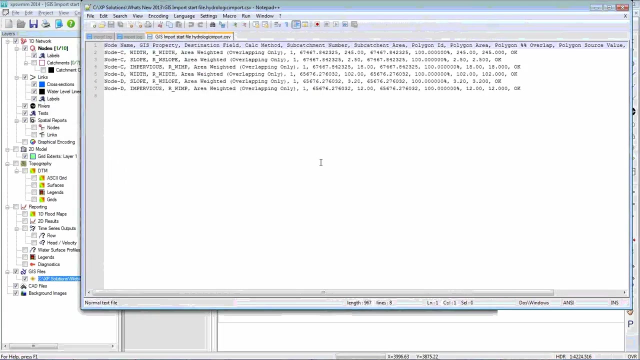 I've only got one to demonstrate that can work And I can add elements such as slope, And I'll go. I'll just maintain with probably the last one that I'll do here: If I hit import here, the software gives me a text file summary of what has been modified. 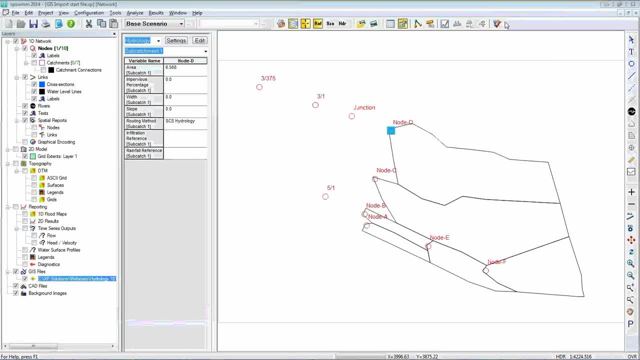 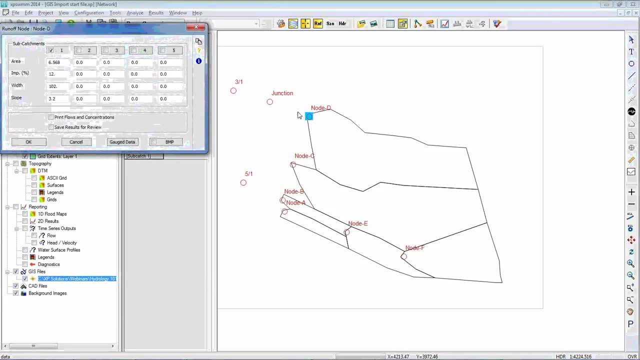 And I can import it, can review that to confirm that the changes are acceptable. But I can also do that inside the software. By double clicking on node D, for example, I can see that I have a fraction of pergis that has been brought in from this GIS file of 12% A width value has been applied. 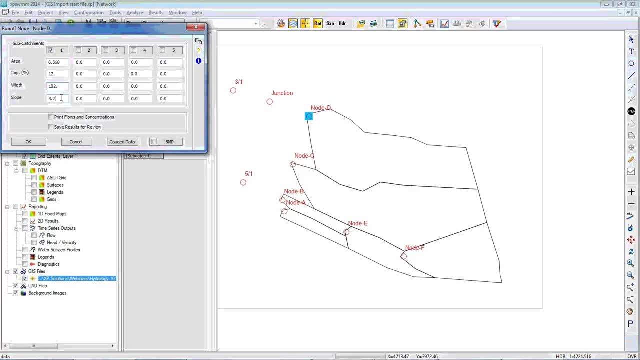 This may be specific to a particular hydrology method And a catchment slope, as a percentage of 3.2% has been brought in from this GIS file, So that's a very rapid way of utilising existing datasets if you have them available to yourself. 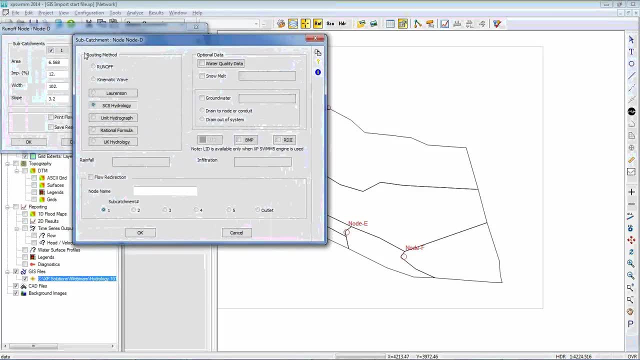 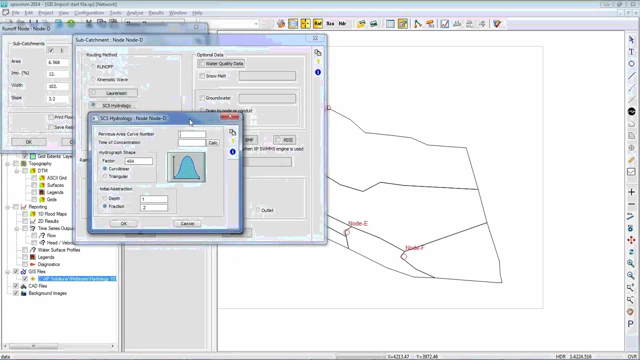 If I go into the catchment, I would then need to tell the software which hydrology method I wish to use. In this example, I'm just going to show the SCS hydrology, And SCS hydrology relies on curve numbers For its loss method And also a time of concentration. The time of concentration could be roughly. 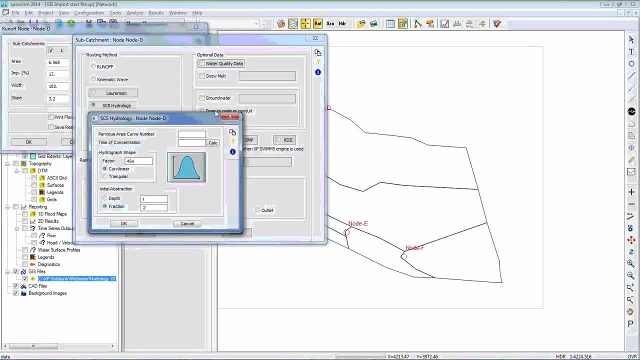 identified based on the length of the catchment, of course, While we're using other calculation methods. But just for today's example, I'm going to assume a 15 minute time of concentration And because I have such a low fraction in pergis, the curve number will similarly be. 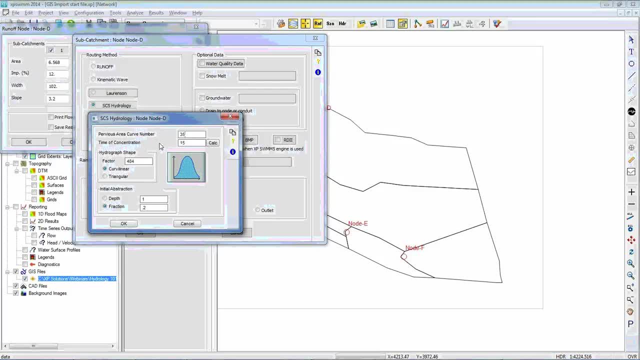 low And I'm going to apply a curve number of 35.. The method also has the ability to have an initial loss or initial abstraction, And I'm going to apply a 10mm initial loss, Again because of the pergis nature of this catchment. 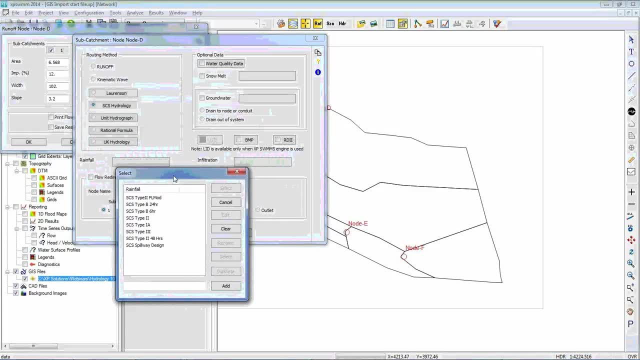 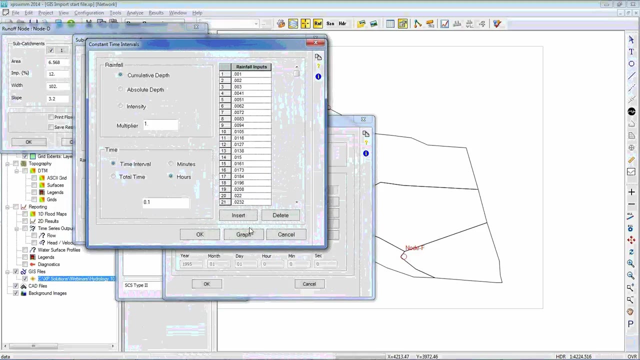 I then have to select my rainfall And I can again use one of the SOAR conservation service patterns. I'm just going to select a type 2 pattern And edit it And I'll show you what that pattern looks like inside the software. And, if I could, graph: 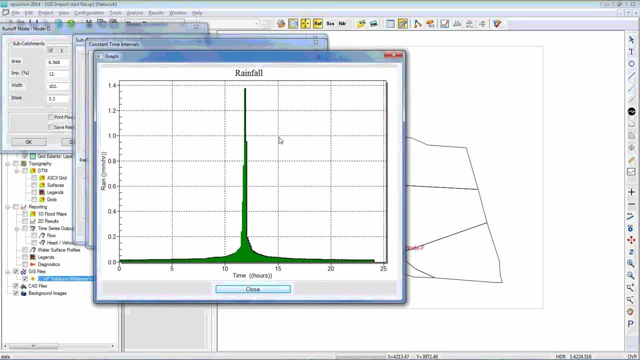 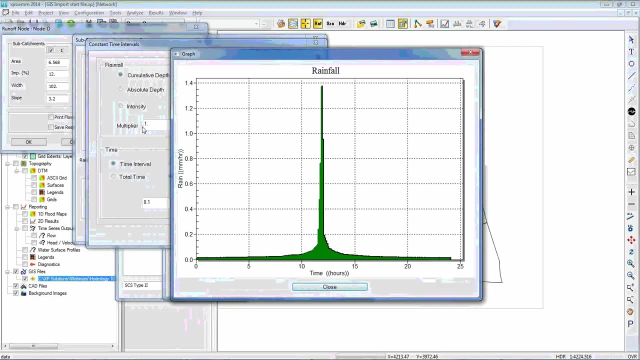 I can see that is the temporal shape of this pattern. We can see here, though, that the rainfall intensity that's currently being applied cumulatively adds up to only 1mm, And that's a function of this multiplier in the dialog box below. 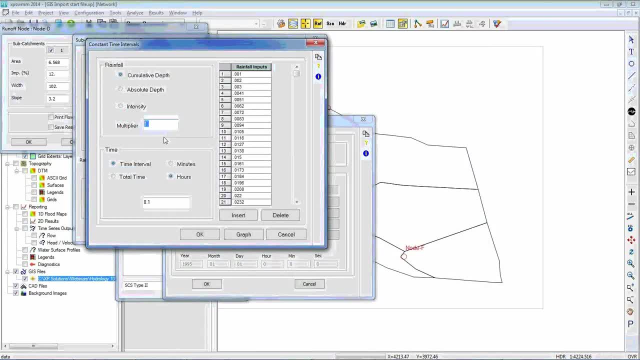 So if I go back to that point and if I were to apply a 24 hour, let's say, 100 year depth or 1% AEP rainfall value, I might expect that to be in excess of 350mm for where I am here. 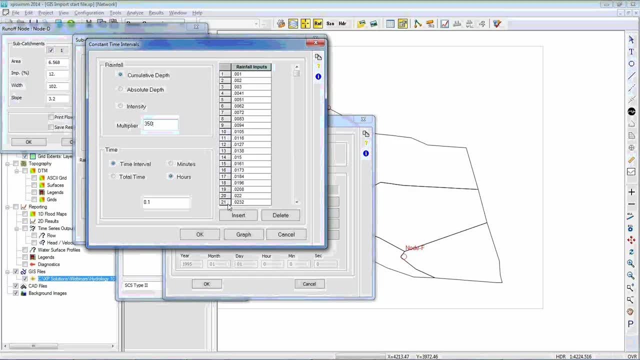 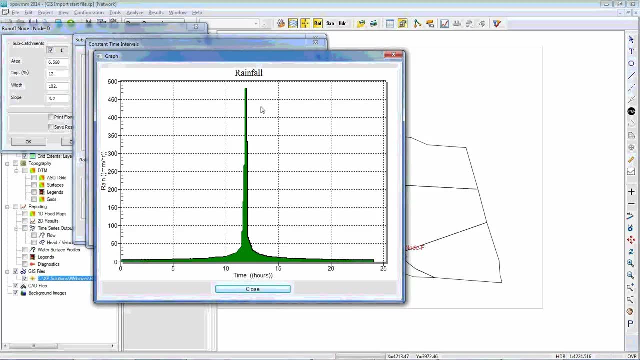 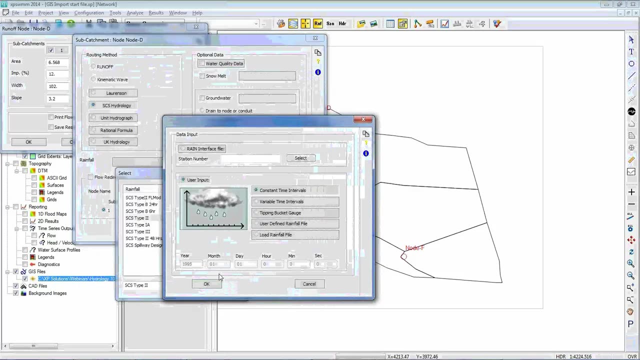 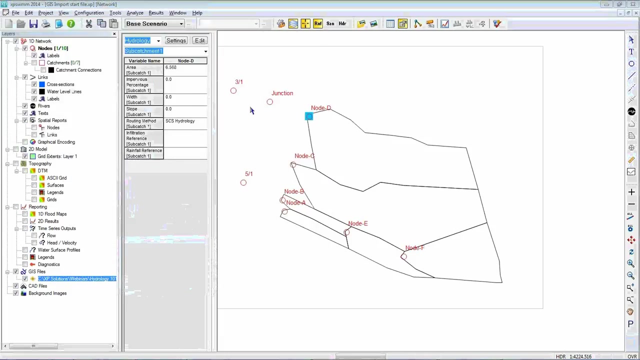 in Brisbane, in Queensland, Australia, And so now, if I re-graph that, I can see that for the peak of this event, I might expect rainfall intensities that nearly approach 500mm per hour. I'm going to hit OK on these elements, select that rainfall and hit OK This information. 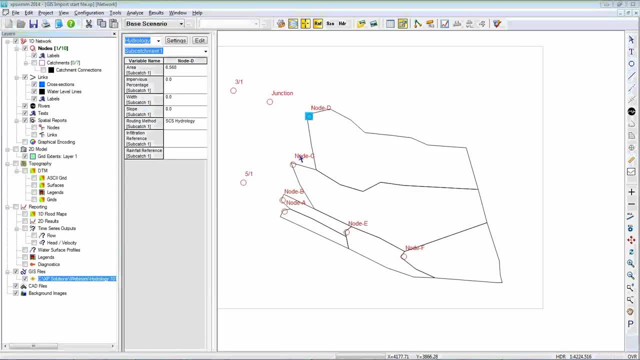 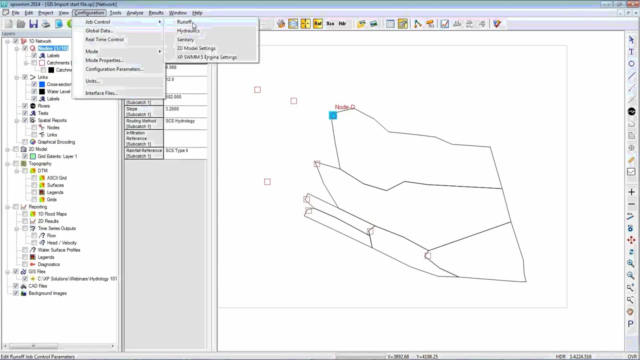 then needs to be transposed to the other nodes inside the model. But just for todays example, I'm going to run that one particular element and just going to turn these elements off before I run the software. But before I do run, even Hydrology also needs to know the time that it occurs. 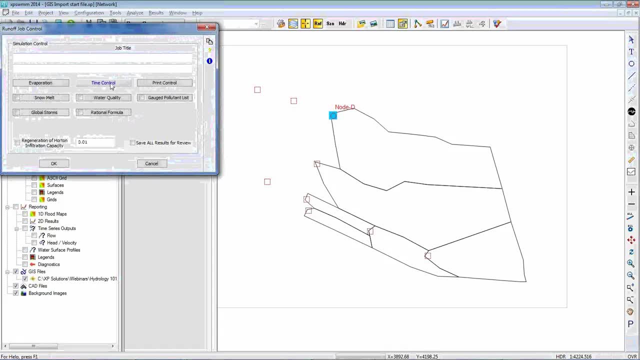 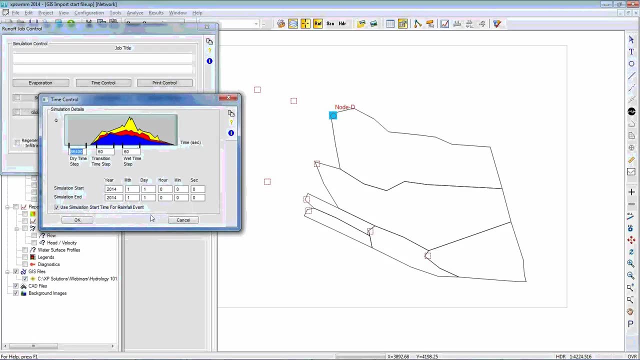 We do this under our Project Job Control. If I go into my Time Control Settings, I'm going to run this storm. I'll tell it, because it's a design event, that the time that we set here will be when the rainfall occurs, and I'm going to run it for 24 hours. 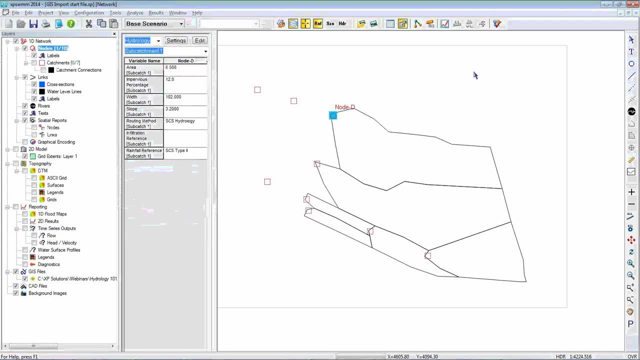 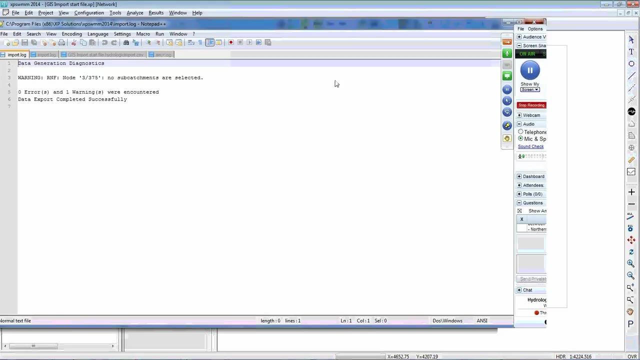 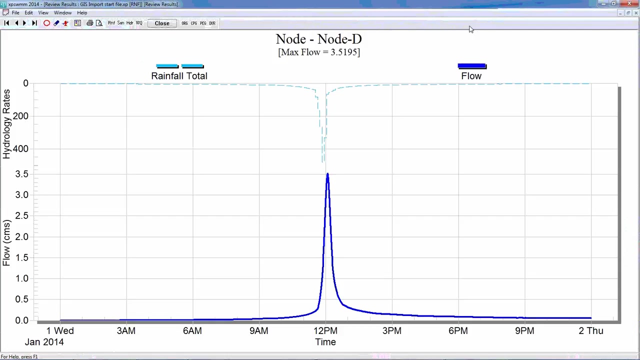 I'm just going to solve this particular model and I'm going to review this particular catchment results. So from this 6 odd hectare catchment I'm generating a peak discharge on this particular pattern of about 3.5 cubic metres per second. 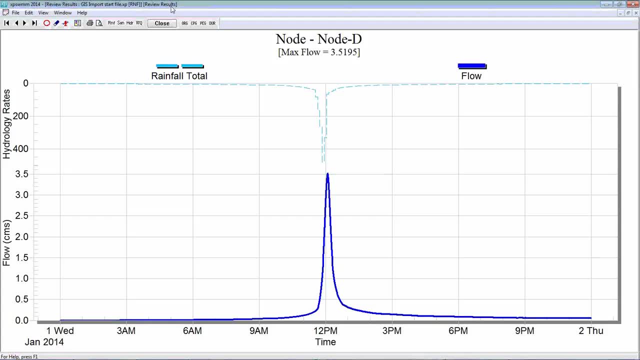 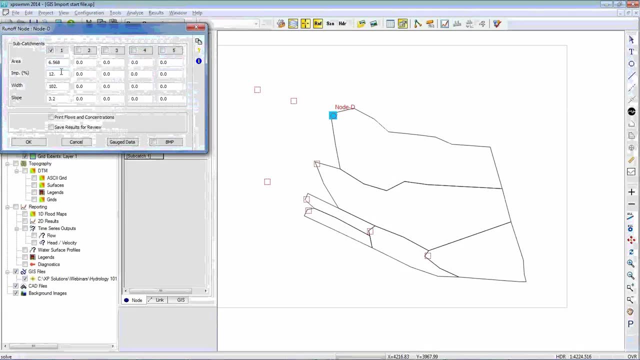 So that's a very simple way of getting our Hydrology results by using our tool, only relying upon the core information, being catchment area fraction impervious, which wasn't actually applied to the SCS method, so that number wasn't particularly important, but also the 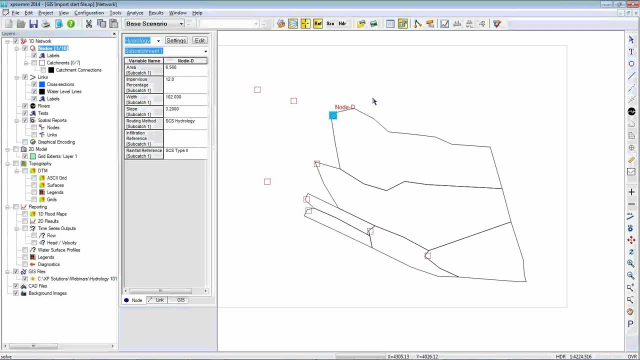 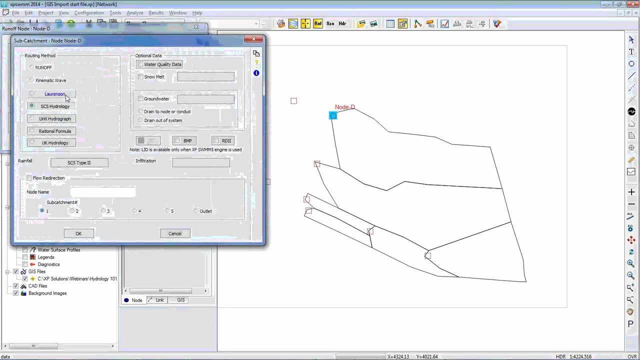 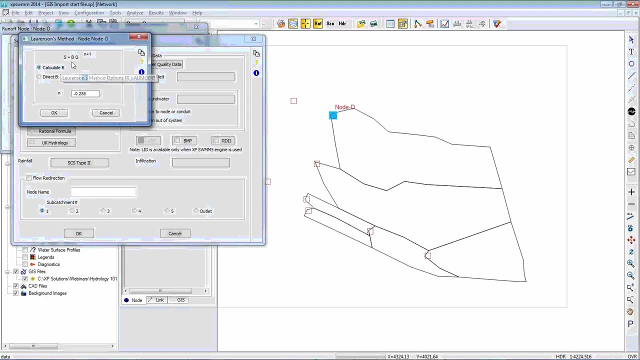 catchment slope, The other Hydrology methods available to us, Which also include, as described before, Lawrenson's method. here in Australia, Lawrenson's method has enough information to calculate the B value, which is the critical parameter for the storage equation. 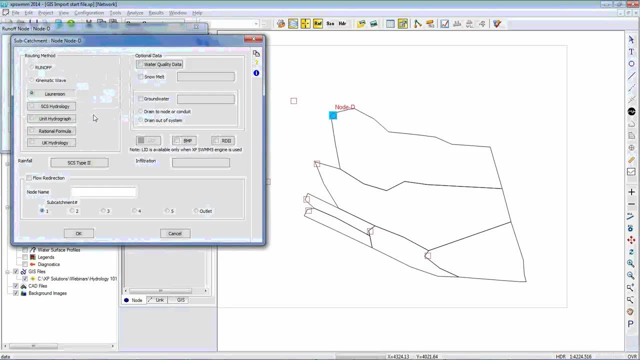 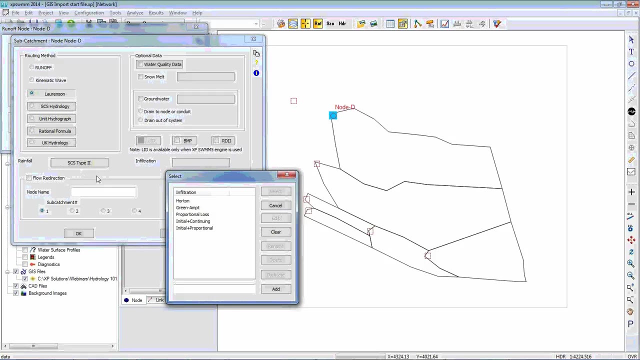 There's enough information inside the software to derive that automatically and we can then select any rainfall. but in that method we would also need to define a loss model, because the SCS curve method has its own internal loss method. One of the common loss methods is an initial continuing loss method. 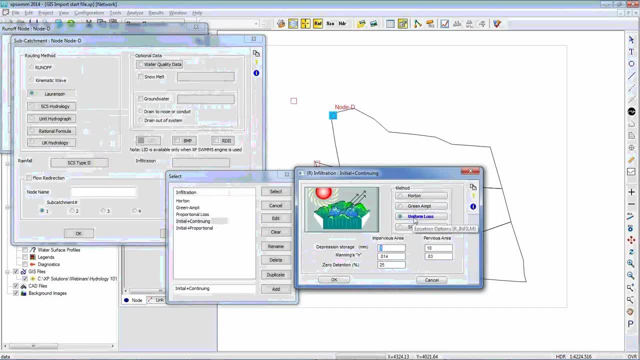 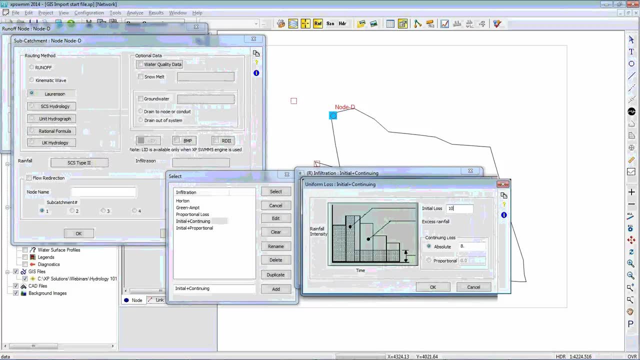 Very popular here in Australia, And under the uniform loss method we can set any value for an initial loss, whether that be 15 or 10, and then a continuing loss, which may be in the order of 2.5 mm per hour. 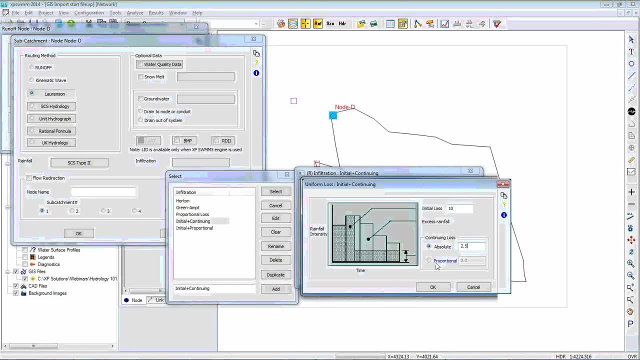 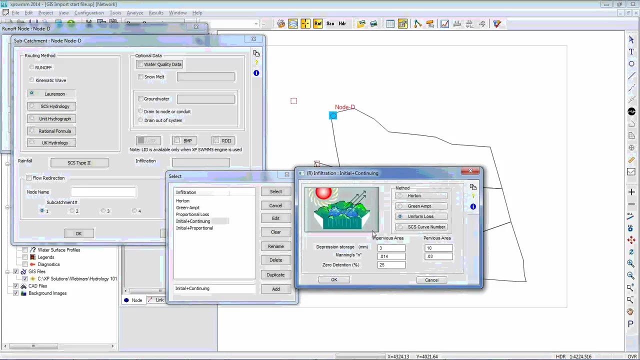 or other As applicable to your catchment, Or, conversely, you could go for a proportional loss, which is a proportional value relative to the rainfall intensity. Different methods inside the software also rely on potentially depression storage, catchment roughness, which Lawrenson's method does, and also groundwater detention. 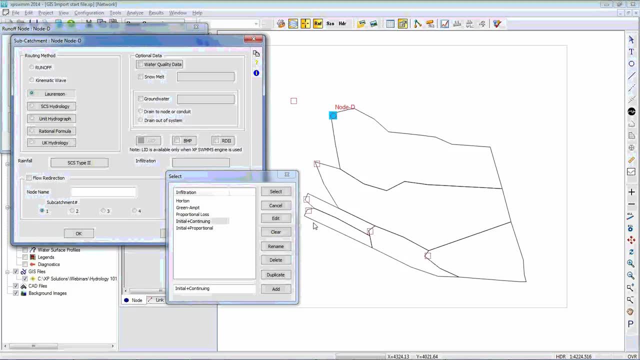 And these need to be specific for each. So what we're going to do is we're going to do a quick summary of the one-dimensional hydrology inside the software And, of course, we could rerun the analysis and generate a different hydrograph. 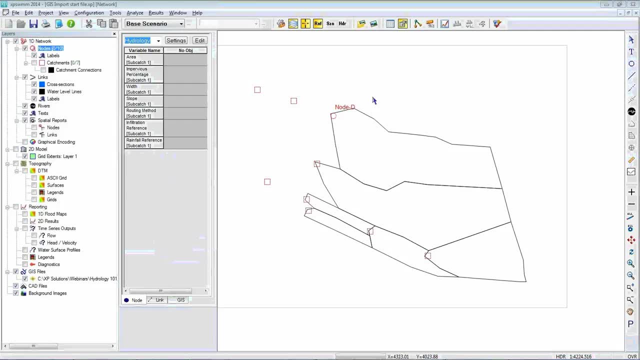 That's a quick summary of one-dimensional hydrology inside the software. However, the other method that is becoming popular is the single-dimensional hydrology, And that's the single-dimensional hydrology, And this is a very common method. It's the one in the past and it's the one that's really popular. 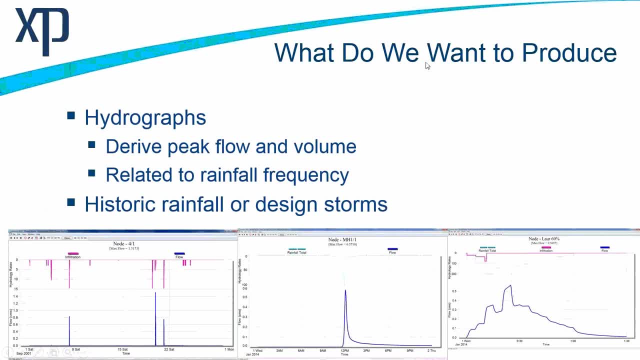 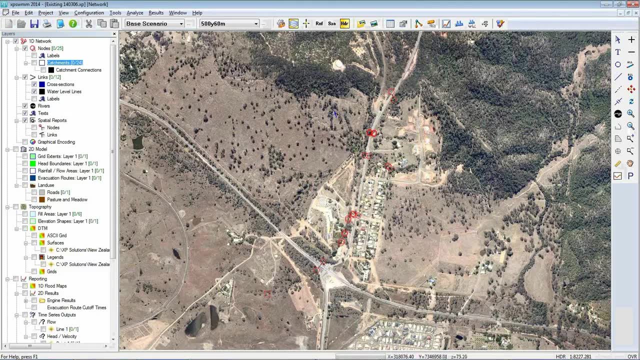 It's been very helpful for Tiburon. I can just click it over here and I can go and select one. This is the single-dimensional hydrologic in the background. There are two here and there's two here. Now, when we go back to the data set, we can actually see how this is different. 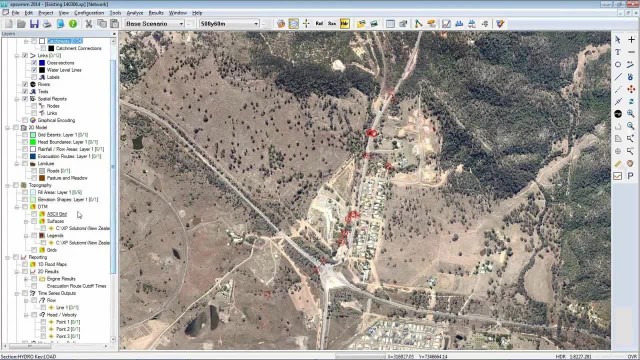 We can see that the one on the left is direct rainfall. So I have another model in the background- I can click over to it- And this is a catchment area here in Queensland. There's two major roadways crossing each other and a small pocket of residential development.